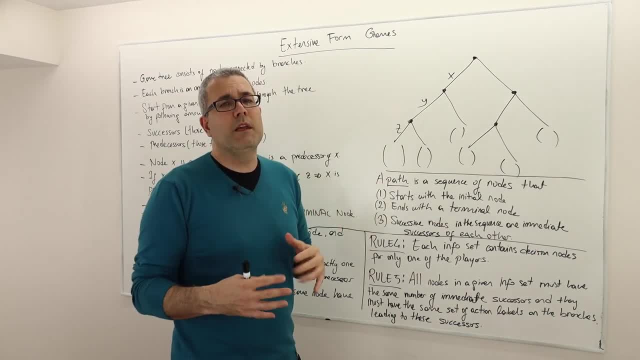 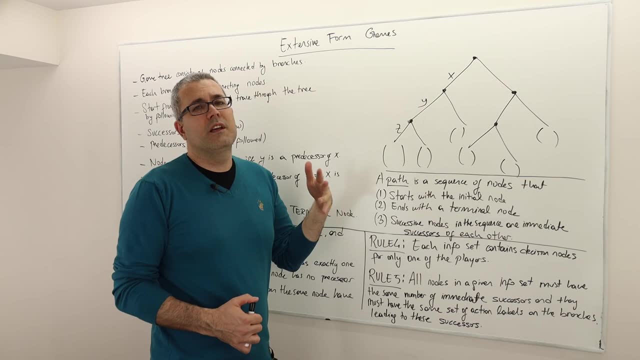 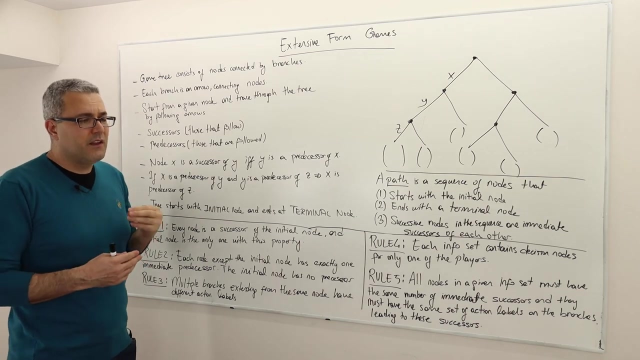 purpose in this episode is to clarify what we mean by game tree. There should be a set of rules, right? Not all tree-like structure is a game tree, So here are the rules. Okay, So, first of well, game tree is nothing but in mathematics what's called directed graph. 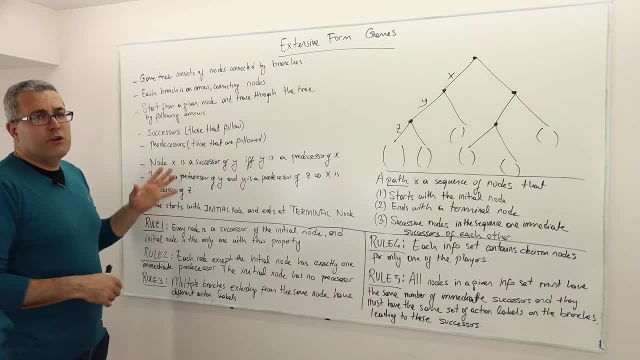 If you, if you don't know what, it is just fine, But if you know what it is, Well, yes, Game tree is a directed graph. Well, game tree consists of nodes that are connected by branches, So this has, for example, 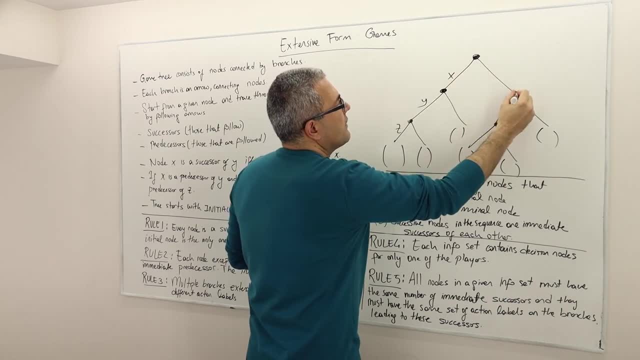 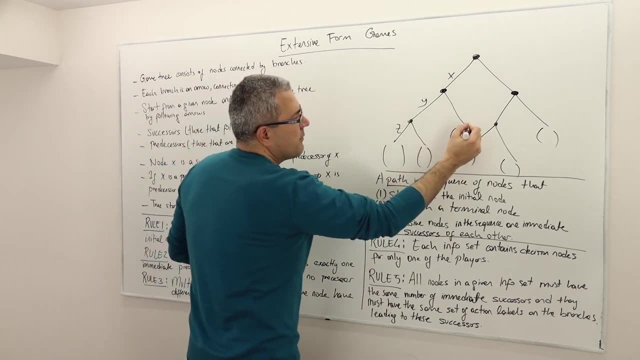 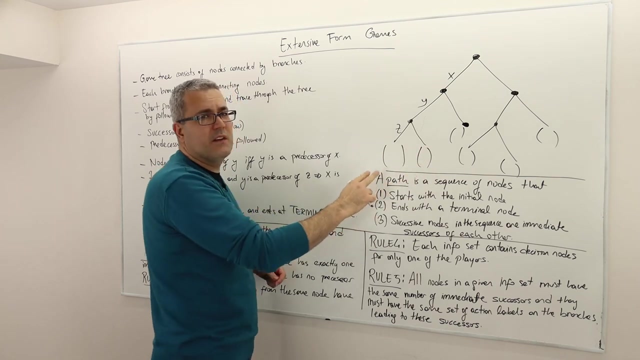 a node, this is another node, this is another node, and those are branches that are connecting the nodes. sometimes this is also called nodes. uh, it's, it's going to be called terminal node. so these brackets are basically the end of the game and and here are the payoffs of the players. 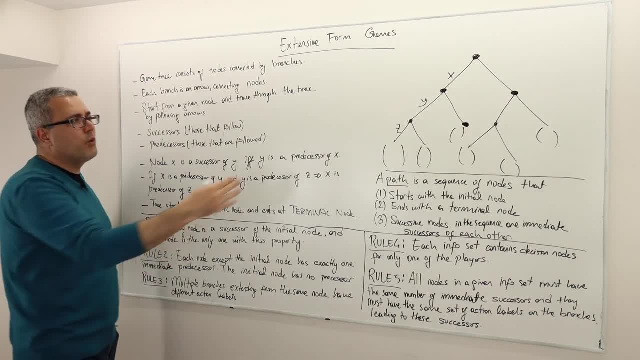 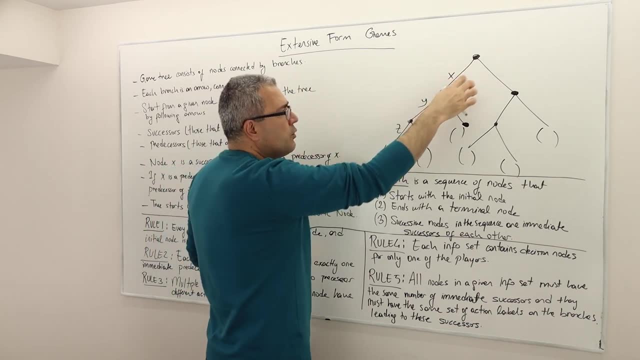 so each branch is an arrow in a sense, although we do not draw them like an arrow, but you can think of them as an arrow. it's a one-way arrow, though, so you always go downwards. there's no upward, uh movement. all right, because that represents the first player and then the 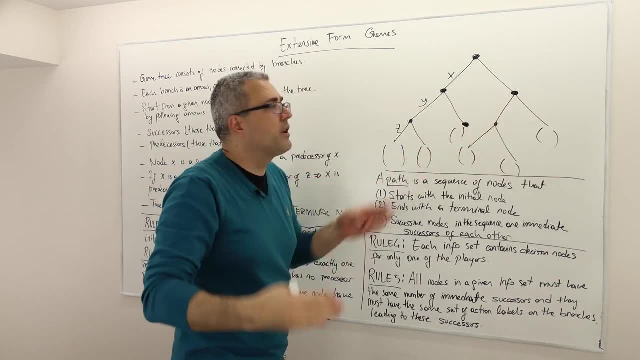 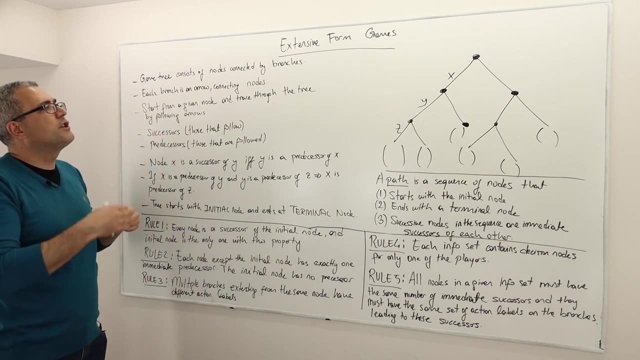 second player or the third player, i mean the, the, the next player in the sequence and then the next players in the sequence, and so on. all right, so each branch is an arrow which connects two nodes. well, you can start from a given node and trace through the tree. 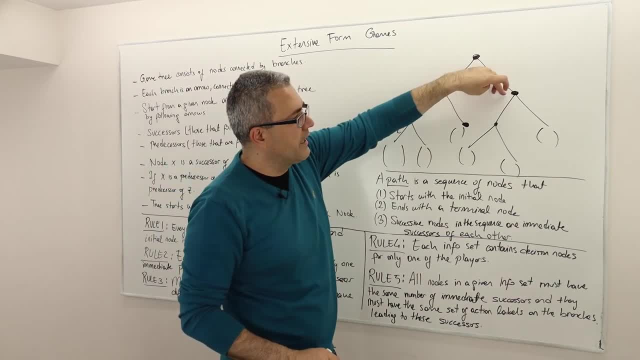 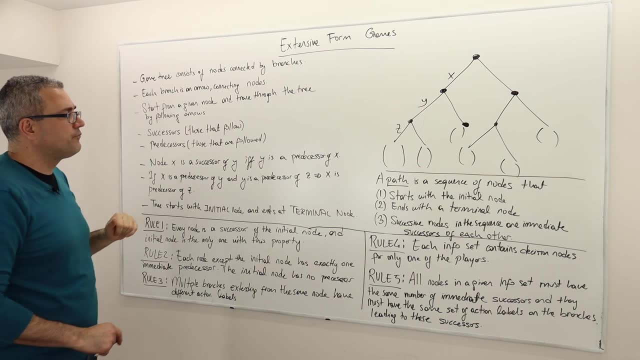 by following the arrows right, so you can start from a given node and trace through all the way until the end of the game. later we're going to call it path, but i'll come to it all right. so the two words which are very important and we're going to use them a lot: successors, predecessors, so. 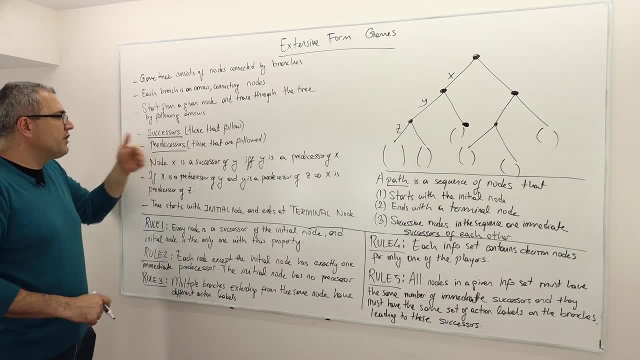 successors are basically those that follow predecessors. so i mean, just remember it from the pre. so predecessors are those that are followed. so, for example, uh in in. you know there's elections in united states, so you can think of donald trump was- uh, it was was the successor for obama and obama was the. 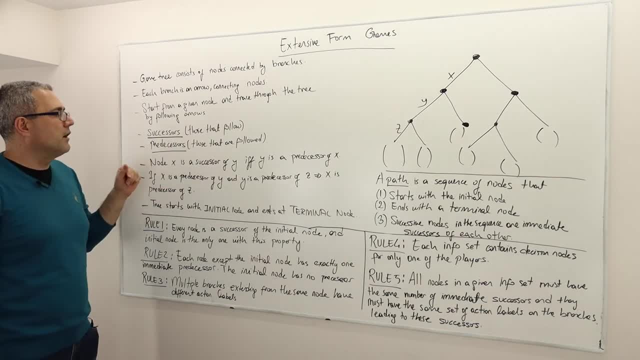 predecessor is the predecessor of uh donald trump, okay, so these words are important. you'll see why. all right, a node x, all right- is a successor of y. if, and only if, y is a predecessor of x, all right. so, if you can, if you think this as x, node x and node y, 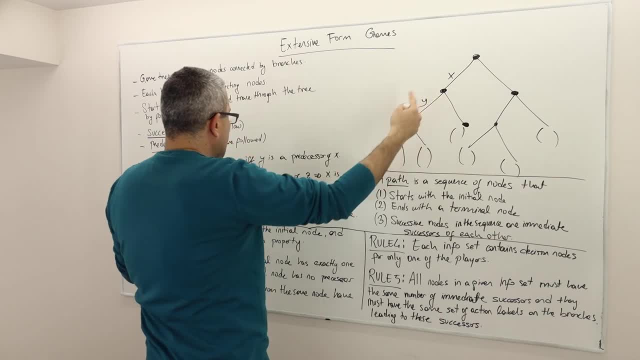 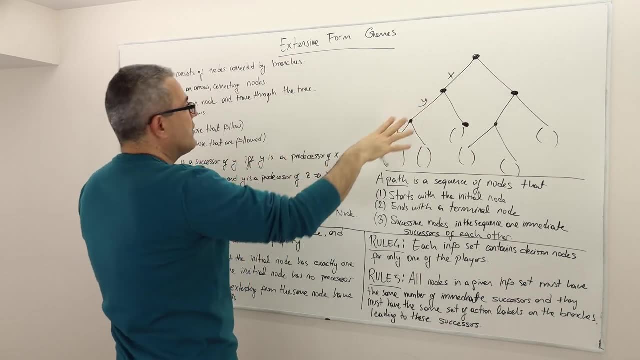 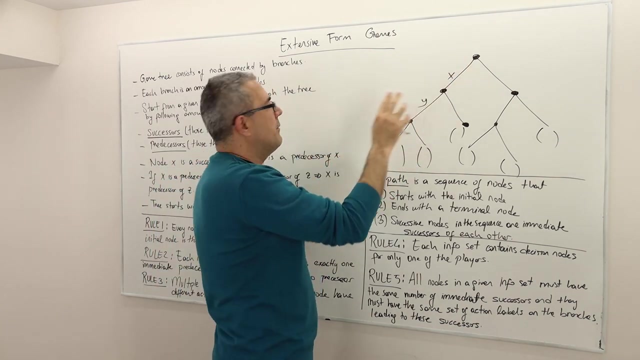 so here x is predecessor of y if, and only if, y is a successor uh, uh, y is a. oh, okay, so here, i'm sorry, the um, the, the x and y has been uh changed. so let me uh. i mean, here x is a successor of y, but here y. 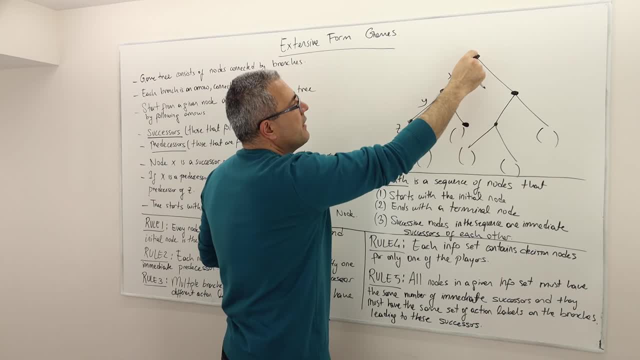 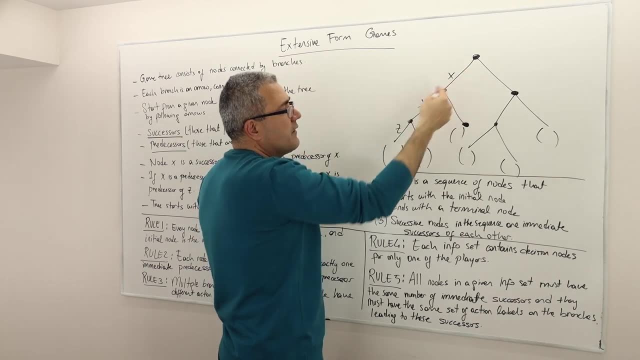 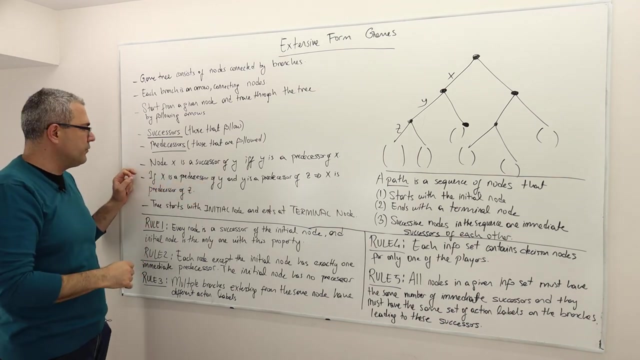 is a successor of x, so be careful about so here. if this is, if this node is x and this node is y, well, and therefore x is a predecessor of of y, all right, so, um, i hope that's clear and i i hope i did not confuse you with this. uh, you know, switch in notation. all right, so if a decision node x, 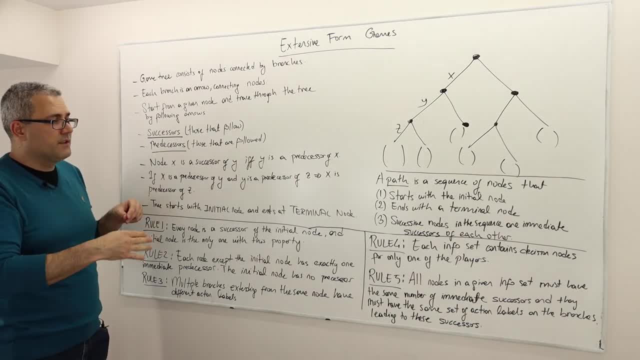 is a predecessor of y and y is a predecessor of z. well then, x must be predecessor of z. all right, so this idea of successor being successor or predecessor is some sort of a transitive relation. okay, okay, well, uh, a game tree starts with what we call. 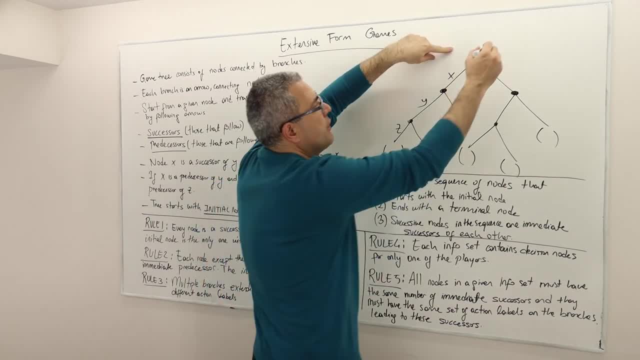 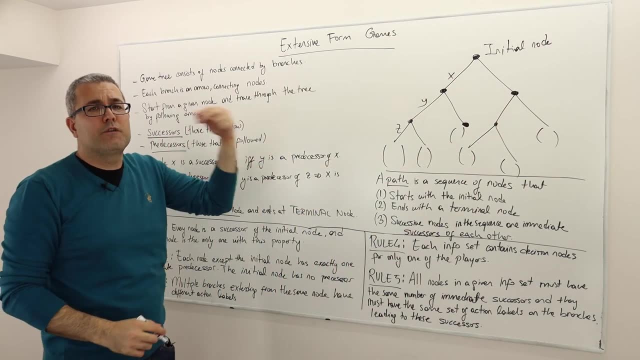 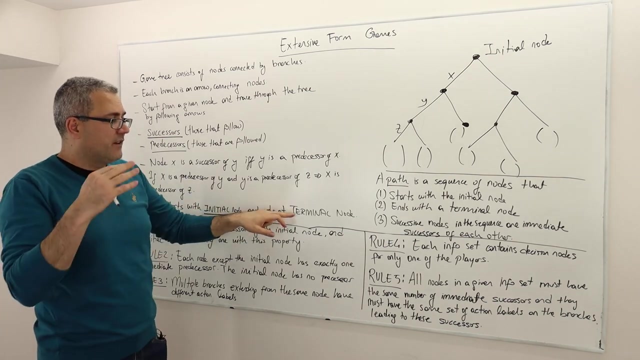 initial node, all right. so, for example, this is the initial node. it basically represents the beginning of the game or the first player that moves in this game, and and then each game, each game tree, ends at some terminal node. so this is a terminal node which, uh we represent, depends on the terminal node we represent, the terminal node which, uh we represent, the 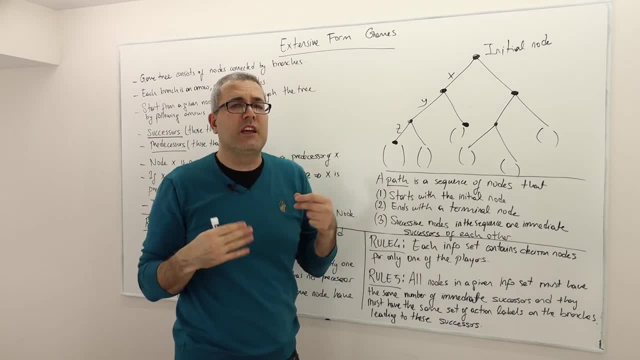 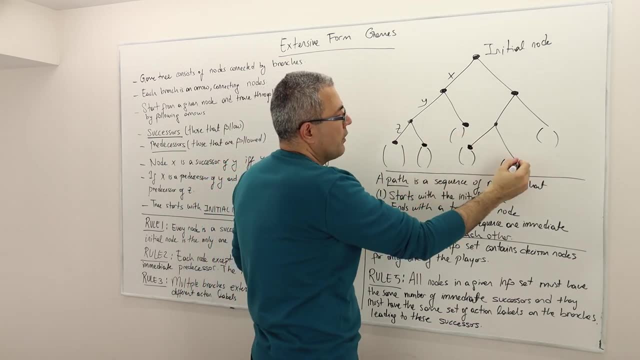 first player, the first player, the first player and the second player is: uh, is the starter node okay, and one of the advantages of these twofenms is that you can say, oh, this node has insan after uoo, which is a debug node, and then this node, because you only have sense data, which is update. 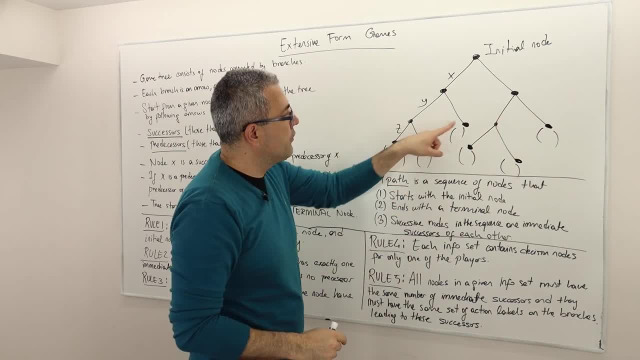 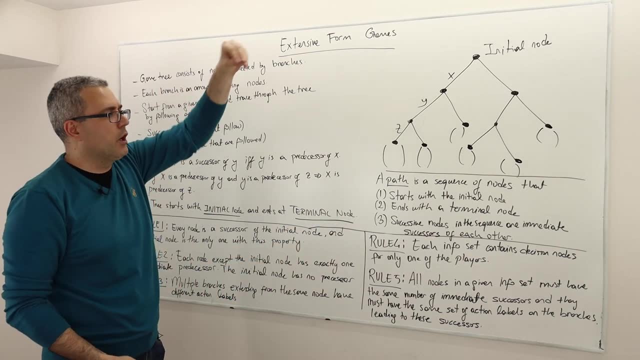 so, again, it's artistic, dying, it's modern because it can work right, and that's a good thing. so what the first player has is is an initial node, and this is our third. we have no node, we have one which is a step node, by a step node which is a step node. uh, so one after. 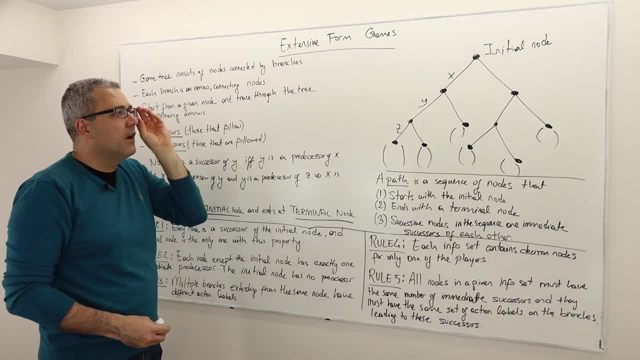 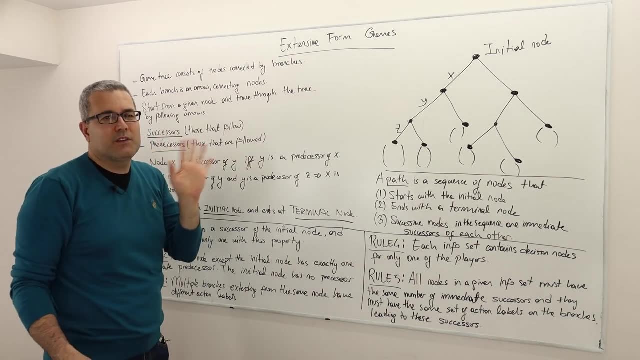 SHA of a sub segment, but it optionally- 돌om 패 is another terminal node, uh, and it can have, uh, some additional actions based on the whole unit from part of it as well, as also it allows us to, but I'm gonna take it back. I mean some, some weird games or some interesting. 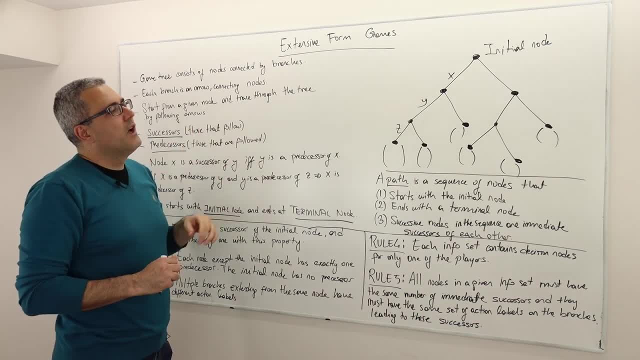 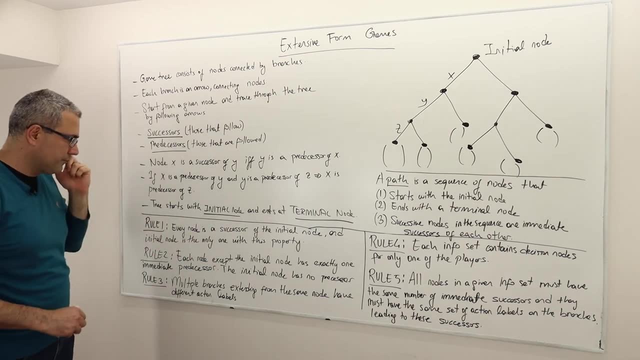 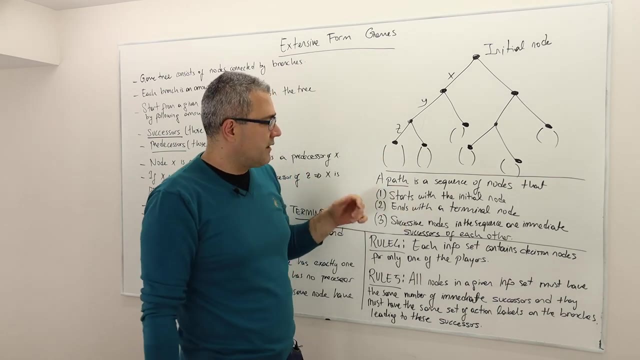 games may have actually two initial nodes, so, but definitely there might be, there will be, more than one terminal nodes. all right, well, what else? a path is a sequence of nodes that has the following properties. one: it starts with the initial node. okay, for sake of simplicity in the arguments, you can 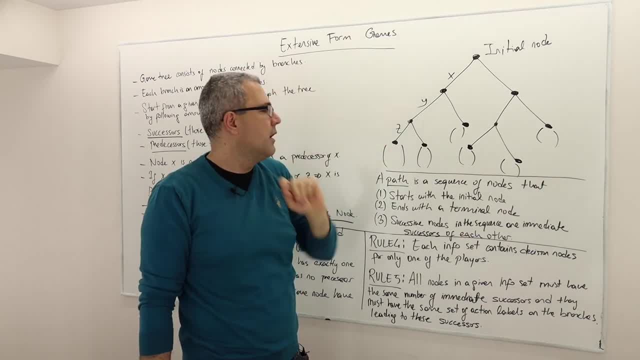 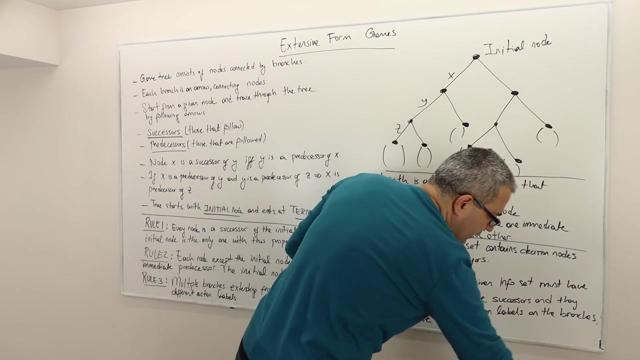 assume that there's only one initial node- okay, a second, the. the path ends with a terminal node and then three successive nodes, in the sequence, are immediate successors of each other. all right, so in this game I'm gonna use a different color. so this is one path. 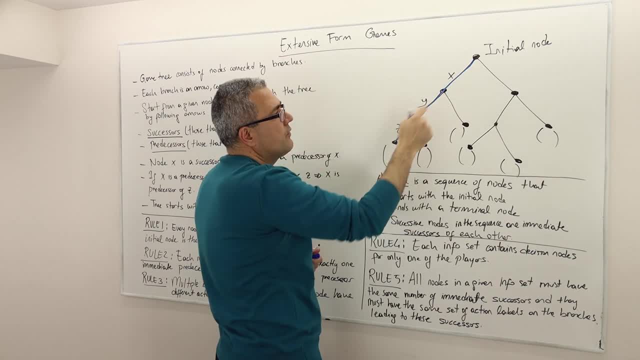 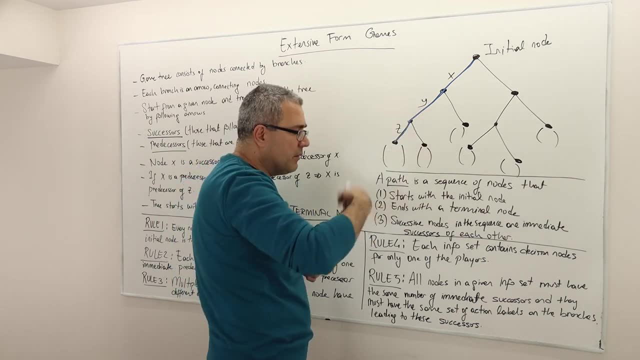 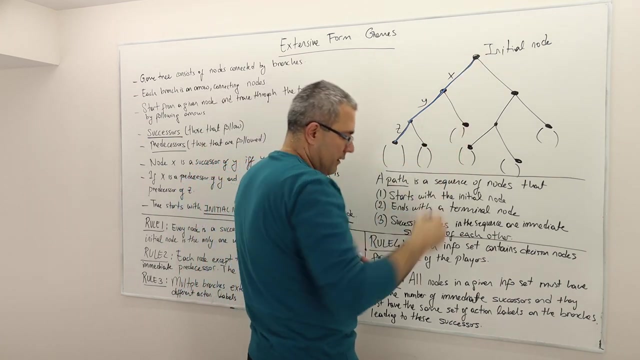 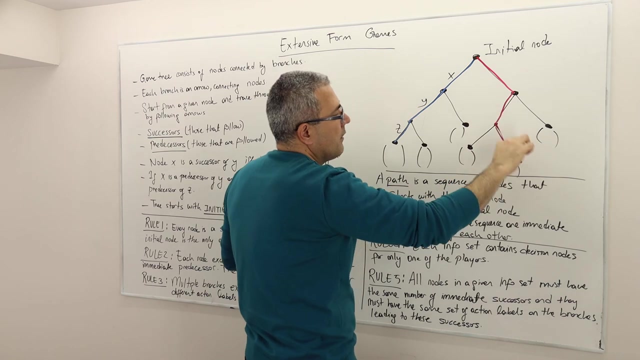 okay, it basically connects three nodes: X, Y and Z. all right, and clearly, Z is an immediate successor of Y, Y is an immediate successor of X, etc. all right, so there are many paths in this game. let me use a different color. this is also a path, all. 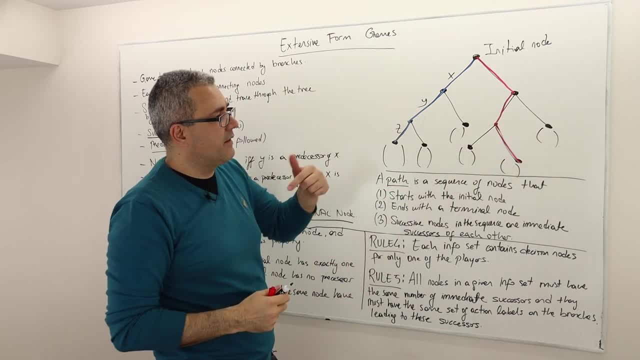 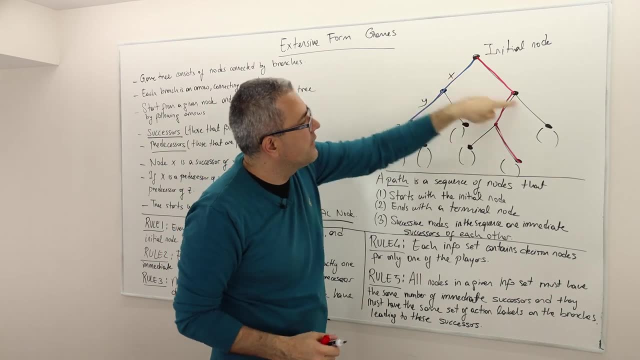 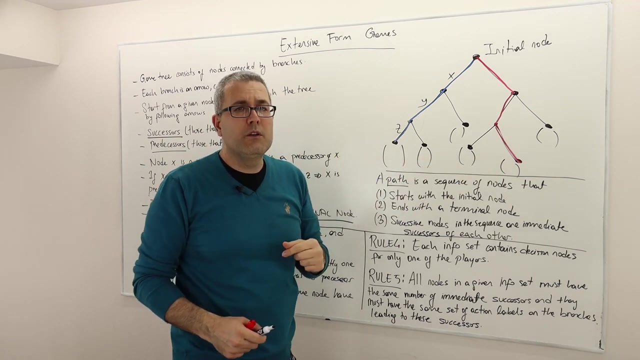 right. so if you count how many paths are there, well, this is one, this is two, this is three, this is four, this is five, this is six, so there are six path. well, is this related to number of terminal nodes? well, yes, normally, and it's. it's what we 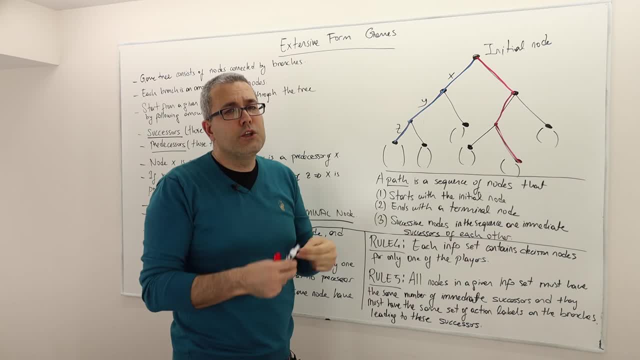 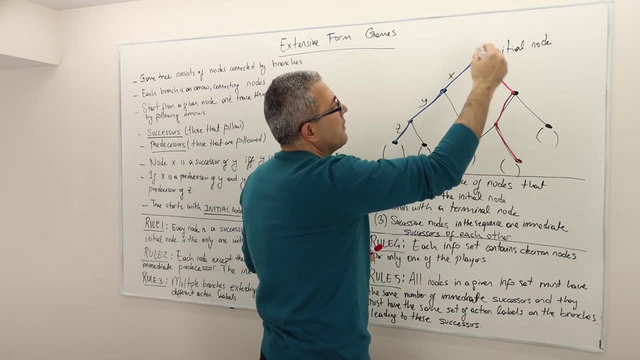 should have the number of terminal nodes determine the number of paths in the game, all right. however, this is not a path, ah. so let's say: we take this and then this, and then another Butow has apathic again. so let's look at, say the we take this and then this. 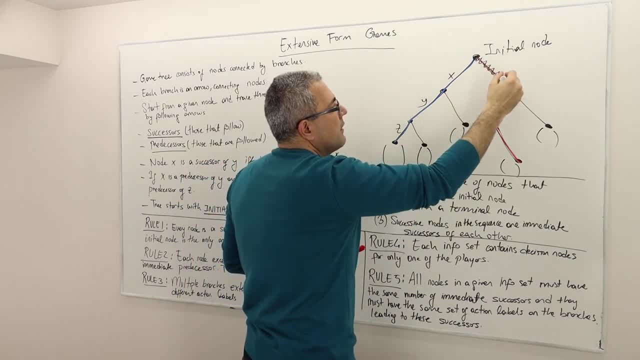 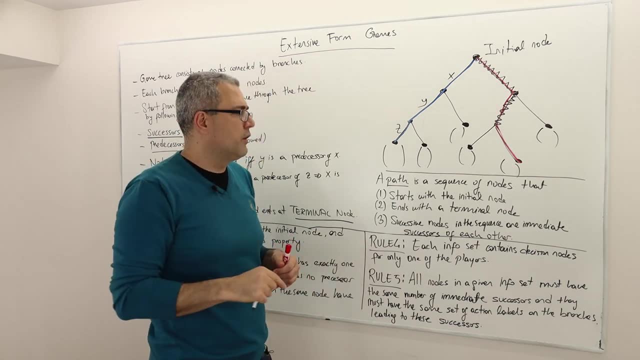 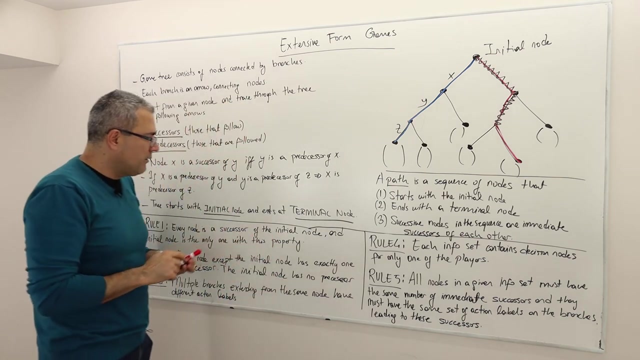 that's it. so this is not a path. so let me. so this is not a path. it's sort of impartial. you have to reach to a terminal node in order to define a sort of path, so it has to be full path. you see what I mean? all right, so now let's. 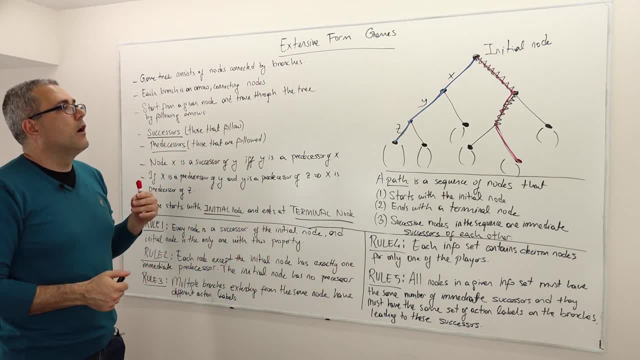 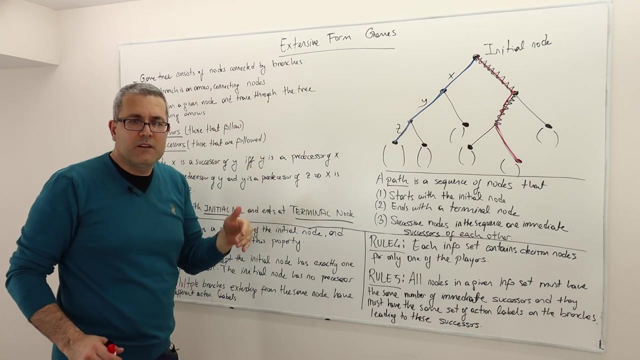 talk about rules. so what are the rules for all these nodes and branches to satisfy and fulfill the concept of game tree? well, rule number one is the following: every node is a successor of the initial node. right, every node is a successor of the initial node. doesn't have to be immediate successor, but 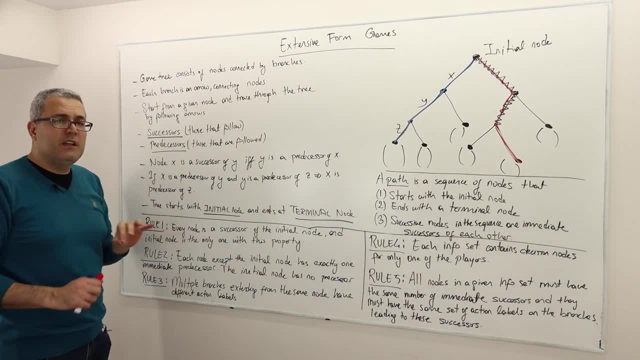 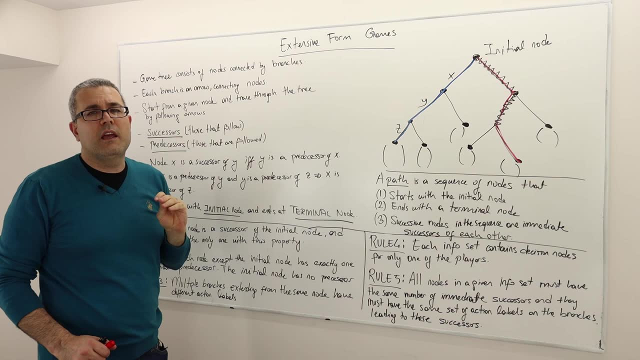 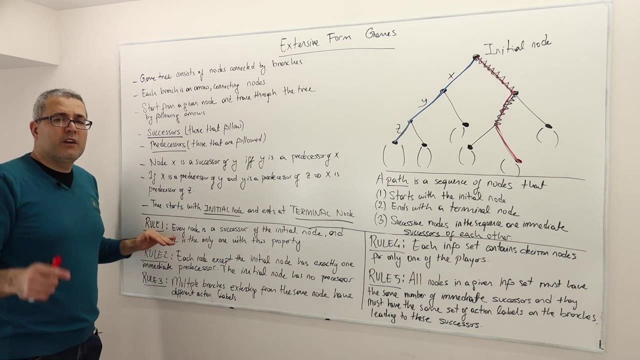 successor nevertheless, and initial node is the only node with this property. all right, so the initial node is not a successor of anything else, any other node, but the initial node, which is the initial node, which is the node which is notes, all right. rule number two says um. by the way, i already posted these lecture notes, so you. 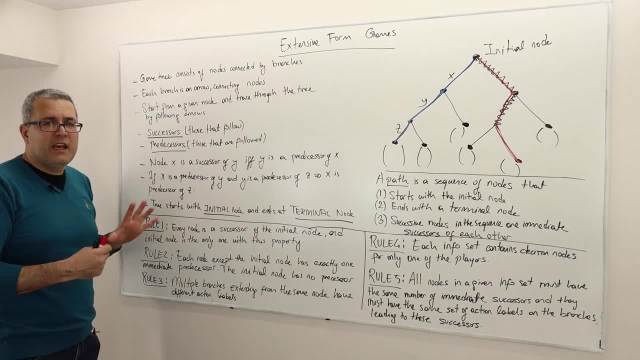 don't, uh, if you can't read them, or if you can't, uh, take notes, don't worry. the lecture notes will be posted on the course website. so the second rule says the following: each decision note- sometimes we call them just decision note, sometimes decision note, so they mean the same thing- so each note. 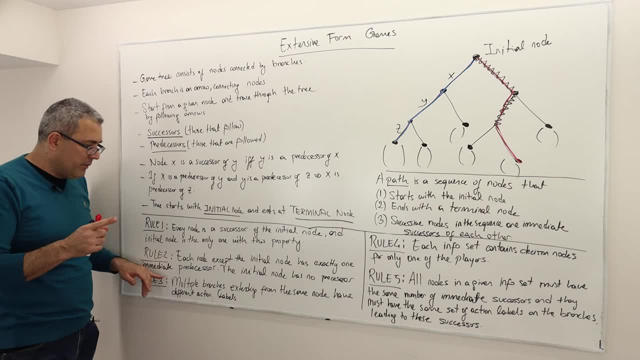 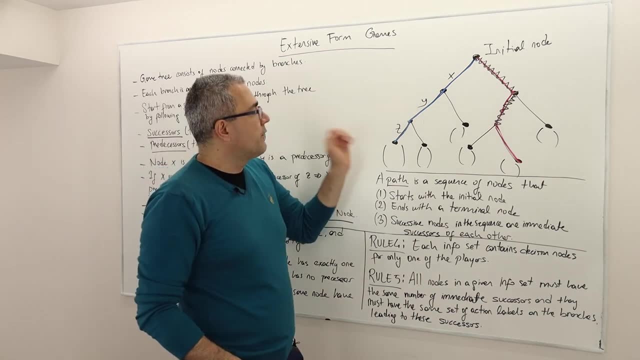 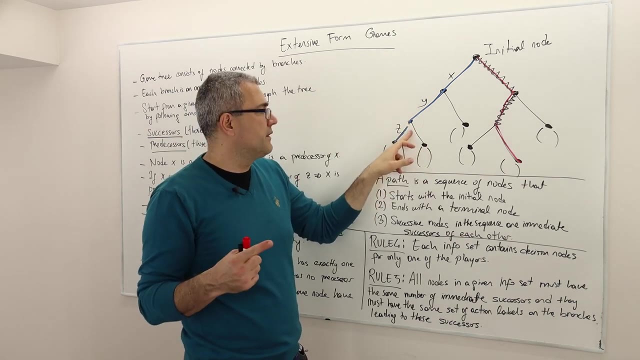 except the initial note has exactly one immediate predecessor. the initial note has no predecessor, so that's very important. for example, this terminal note has only one immediate predecessor, which is z. this also has one immediate predecessor, which is z. again, that's fine, but the thing is, you cannot have. 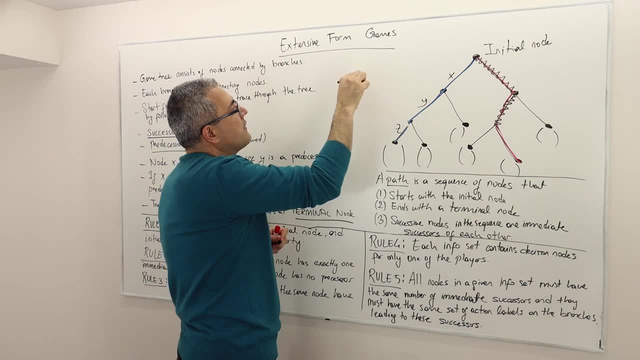 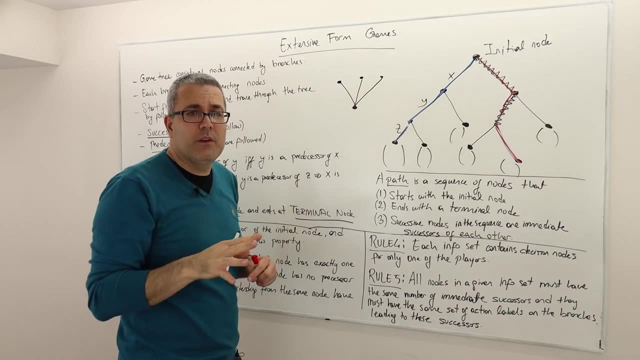 for example, a note here, and it's it has predecessors. uh, immediate, it has three or two predecessors. this can't happen. all right, any, any structure, a tree structure satisfying something like this, will not be, uh, will not be game tree, all right, okay, what else? rule number: 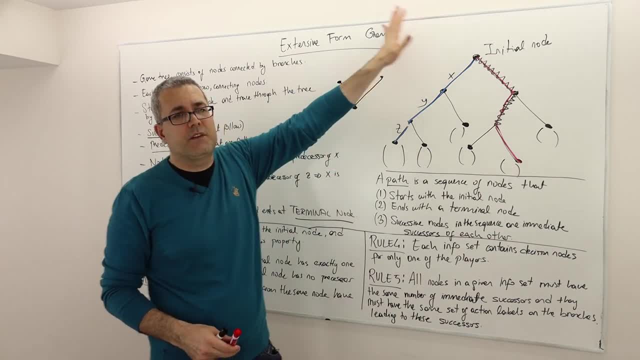 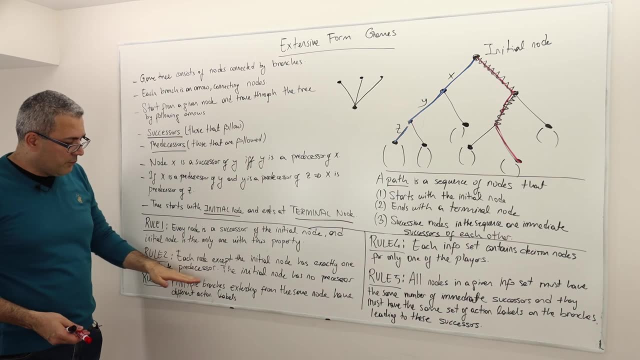 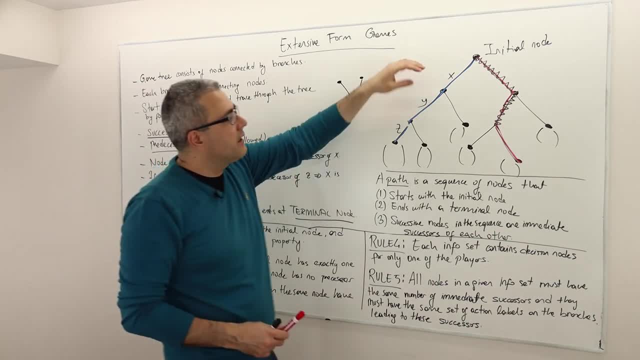 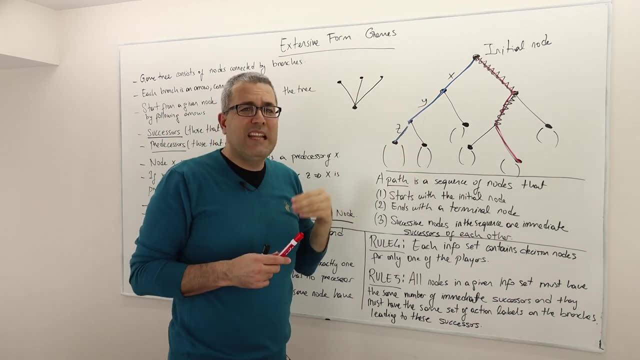 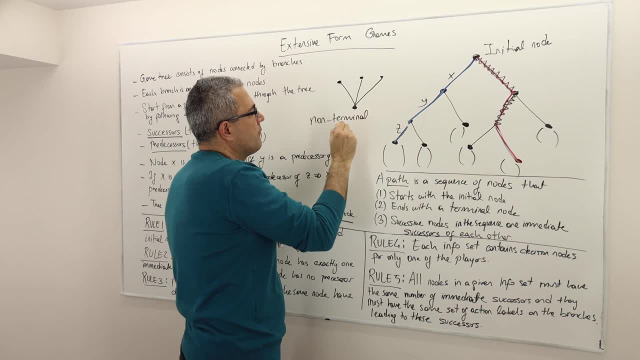 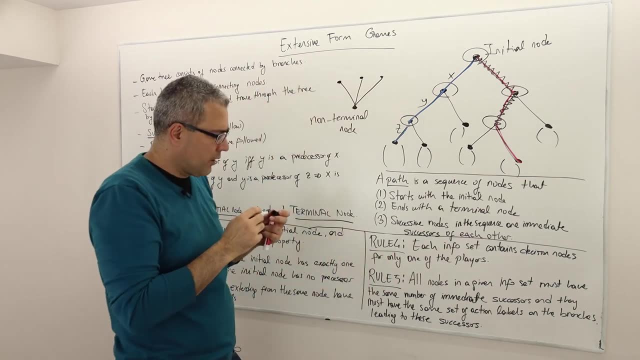 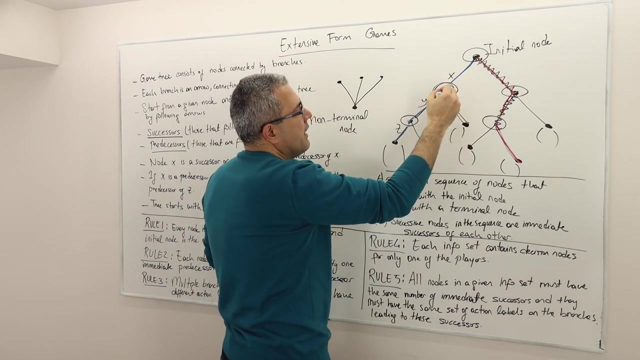 non-terminal node. so here in this game we have one, two, three, four, five non-terminal nodes. okay, so for any non-terminal node there's going to be a bunch of branches, right? for example, this one, this guy has two branches. uh, this guy also has two branches. 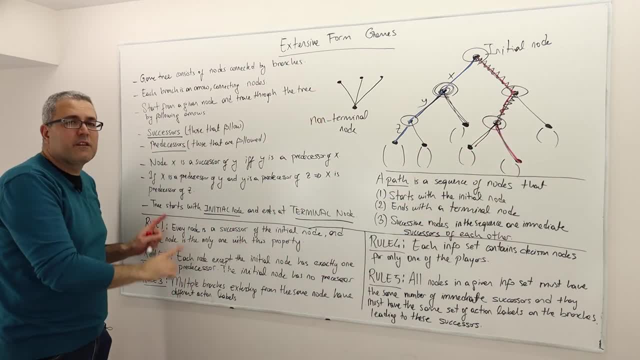 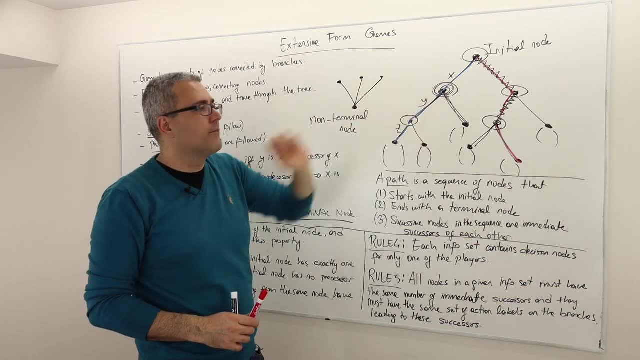 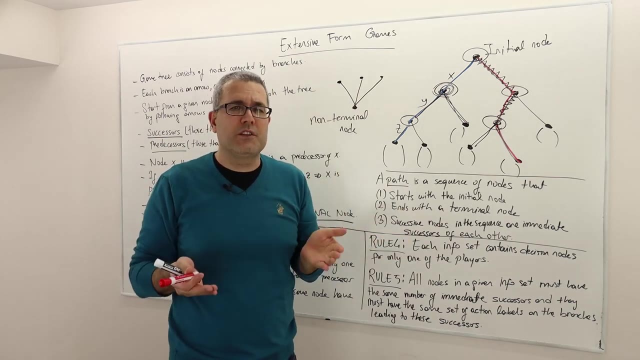 those branches basically tells us: uh, you know the different action, uh that that are available for this player to select. okay, rule number four says each information set. so we know what information set we in in our earlier uh sections and videos we talked about information set. so we 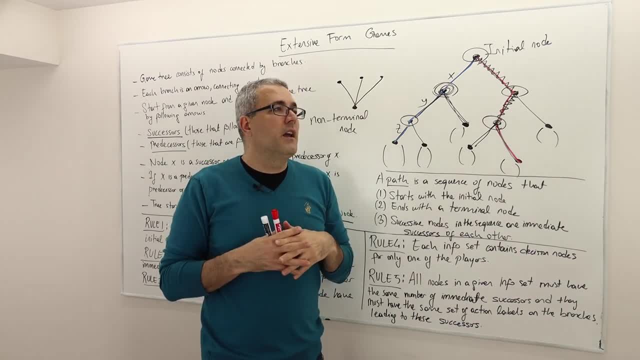 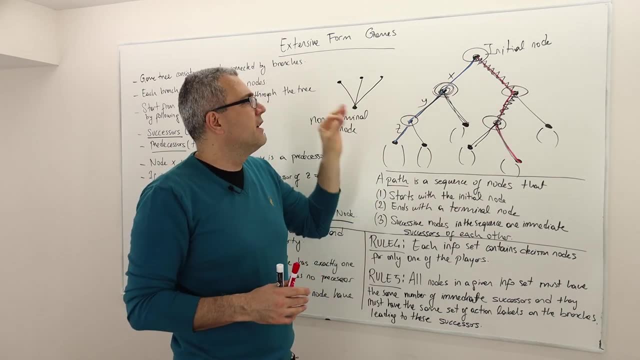 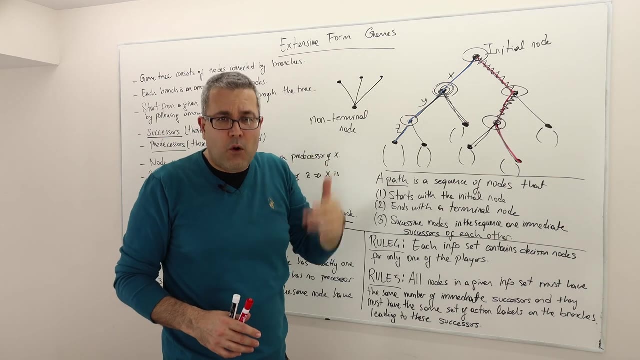 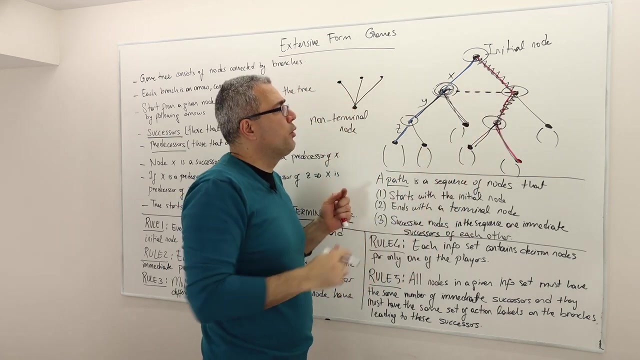 know what information set basically information set is? uh, it consists of at least two decision nodes. so here um, all information sets have single decision nodes, all right, so each non-terminal decision node is also an info set, information set. however, we may have something like this: you know, some textbooks puts dots, some circle them. it basically means these two. 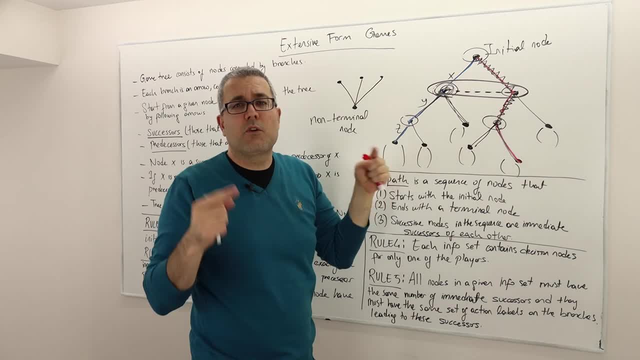 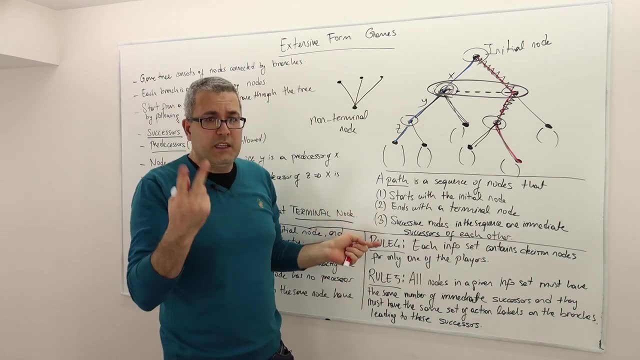 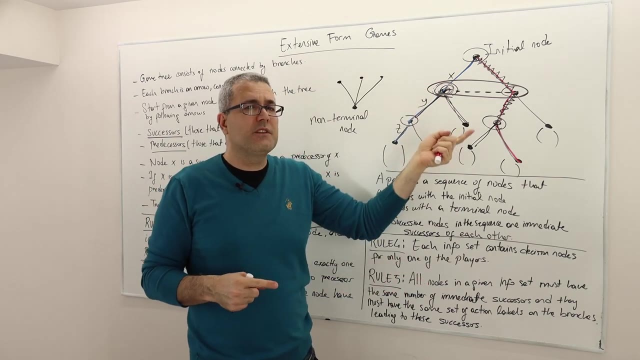 decision nodes are in this information set or are this are in the same information set? all right, so each information set contains at least two decision nodes for only one of the players. what does that mean that means for any given information set, you cannot have nodes that belong to two or more. 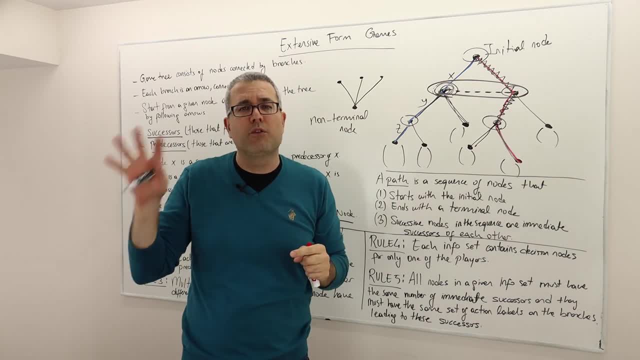 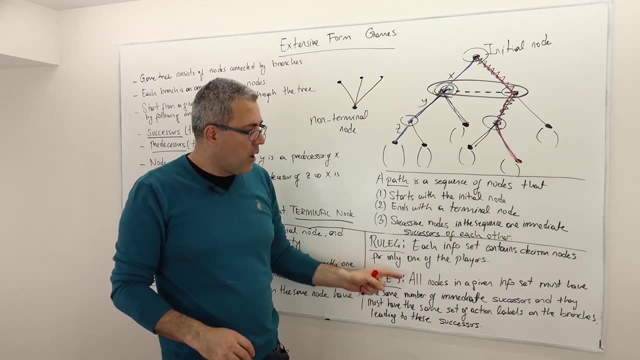 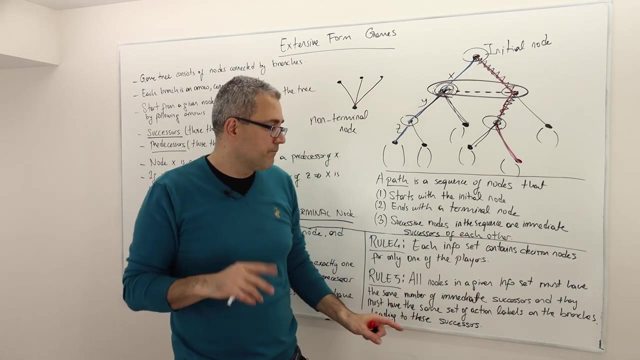 people it has to. i mean all the decision nodes must belong to one and only one player. okay, rule number five and our final rule says the following: all nodes in a given information set must have the same number of immediate successors and they must have the same set of action labels on the branches. 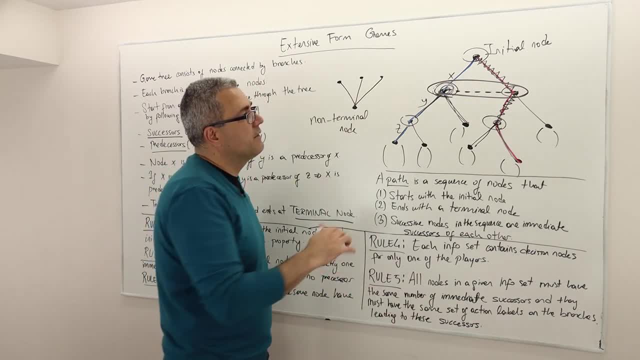 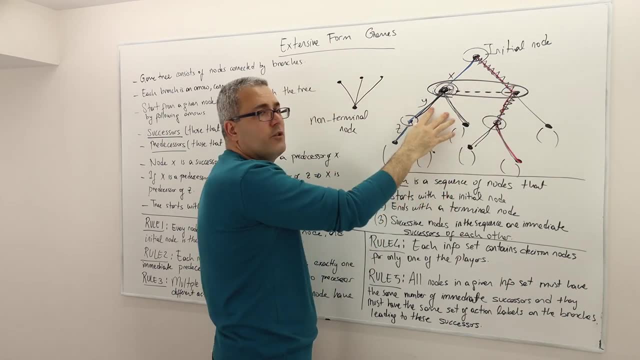 leading to these successors. well, it basically says the following: if these two decision nodes are in the same info set, well then we have to have two branch. if we have two branches here, we also must have two branches here. i mean, if we have two branches here, we have to have two branches. 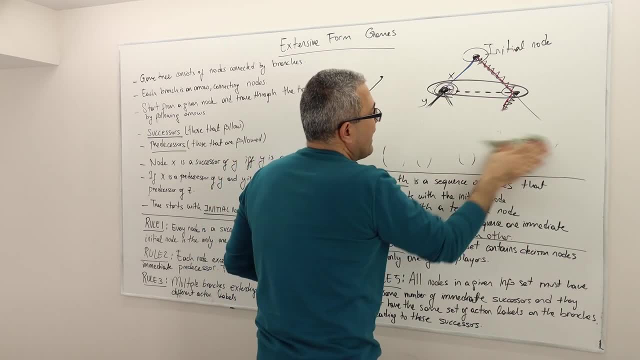 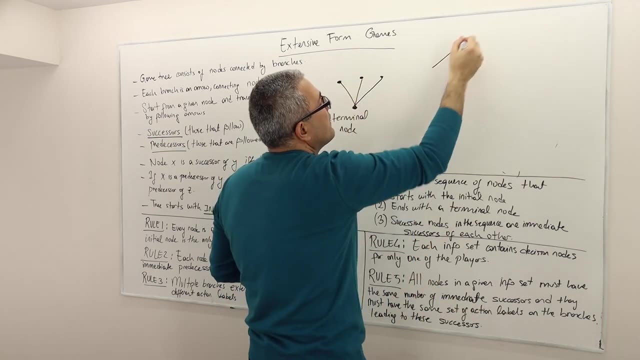 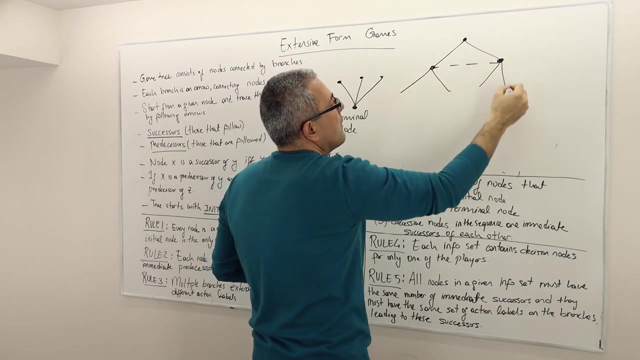 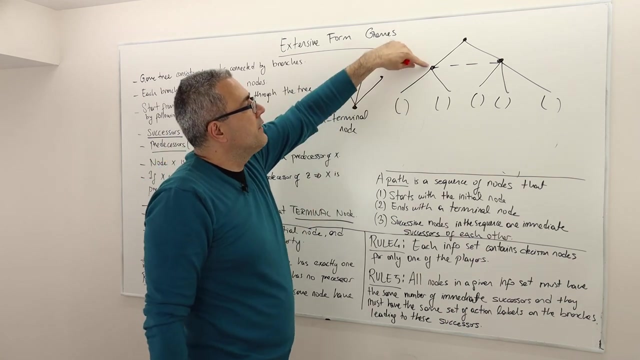 i mean, this is, for instance, not a game tree. very quickly another example: so this is initial node. let's say this: these two decision nodes are in the same info set and the game is over, so the payoffs all right. so this is not a game tree if this and this 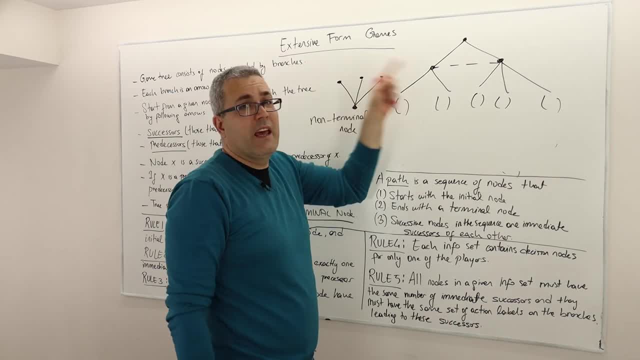 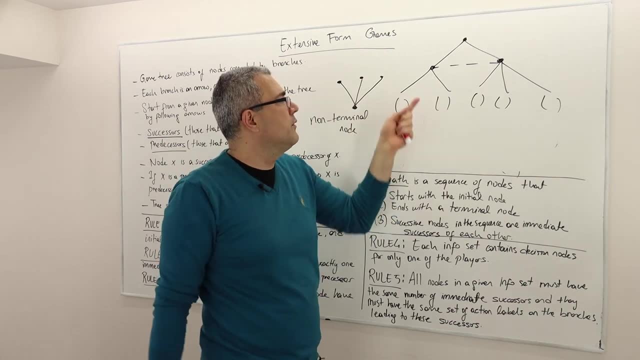 decision nodes are in the same info set, which are which they are. well then, the number of branches that follow these decision nodes must be the same. if you have two here, you must have two here. if you have three here, you must have three here. okay, so let's suppose. 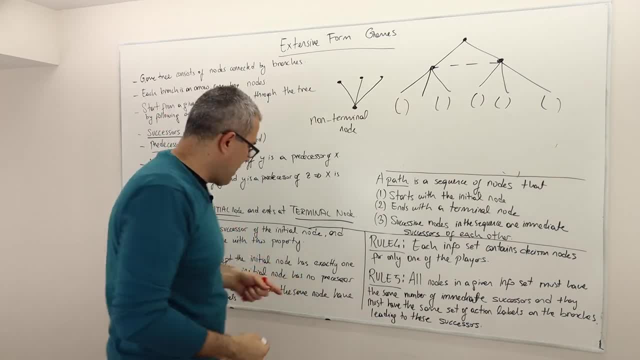 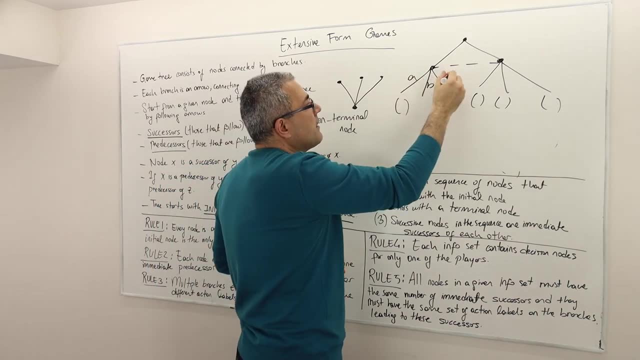 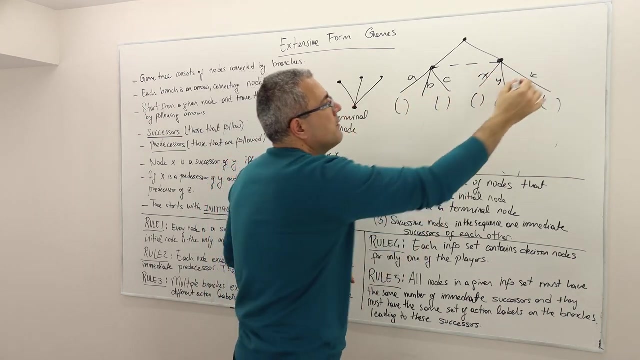 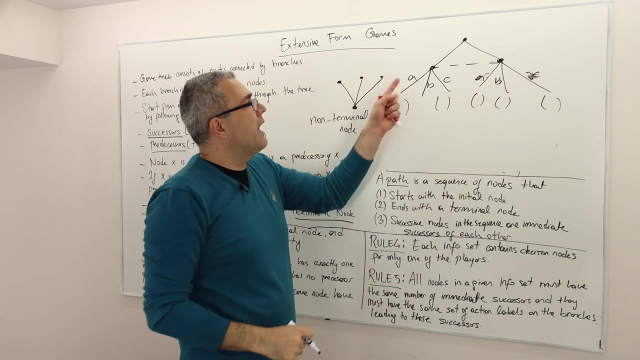 both decision nodes has three branches. that means, remember, branches are sort of different labels for available actions, and if here the available actions are called abc, well, here you can't call them x, y, z, also Z. They also must be called with same letter, all right, A, B, C. So here A means, for example: 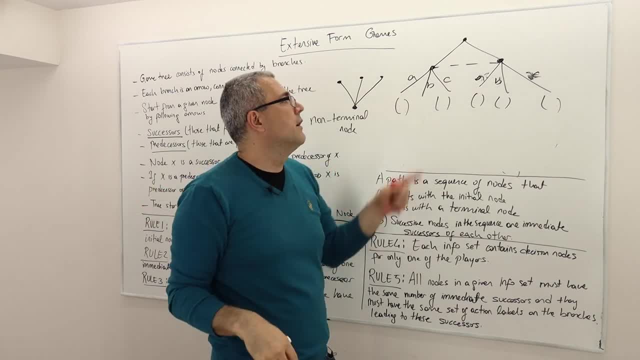 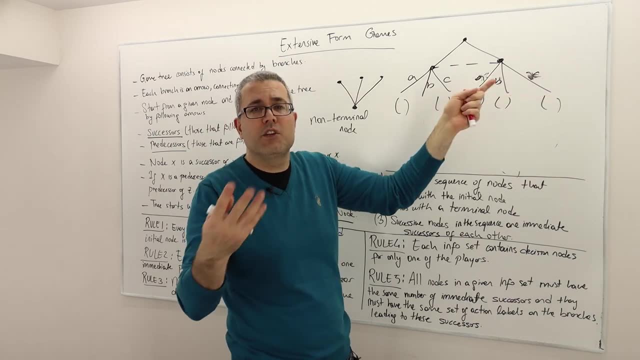 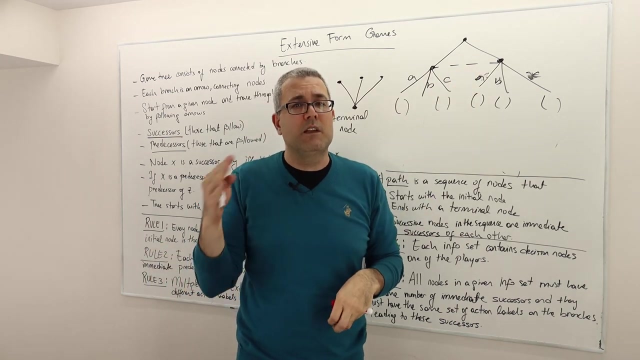 jump up. Here B means hide away And C means scream. Well then, here that means one of the actions available for you is screaming, one of them is jumping, the other one is hiding out. You see what I mean. So the set of available actions in each decision nodes must be the same. 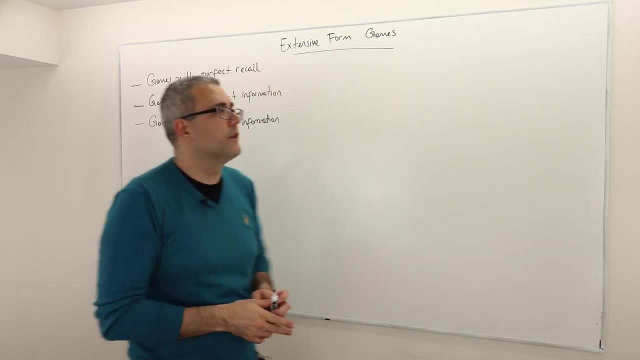 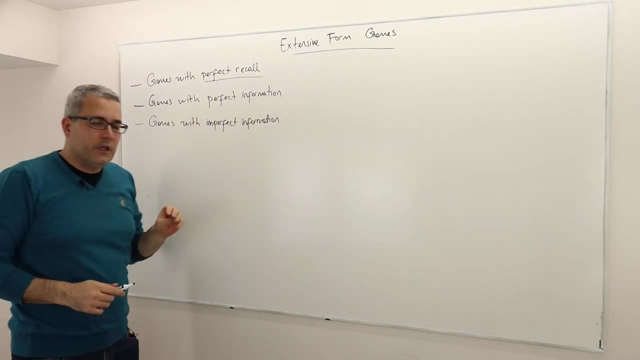 okay, Three notions are important. The first one is the idea of perfect recall. So we are actually talking about, in this course, games with perfect recall. What does that mean? It means all players can perfectly recall all their own previous actions. They may not observe. 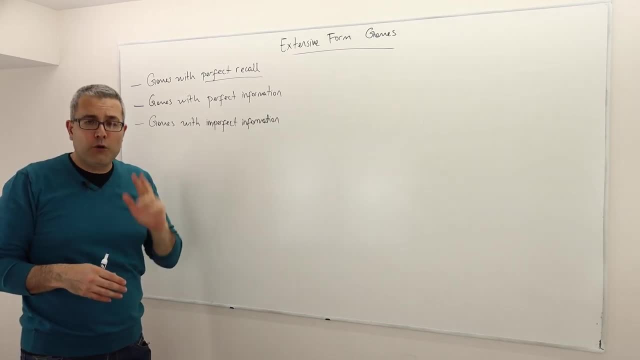 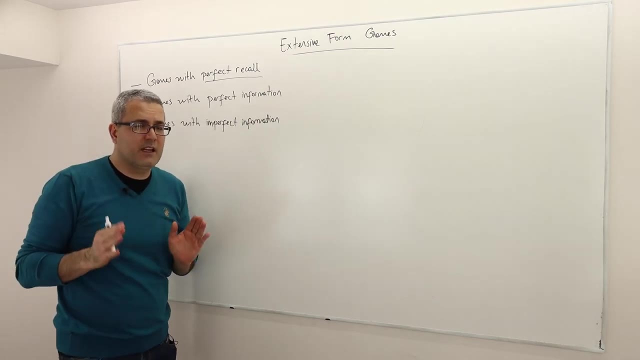 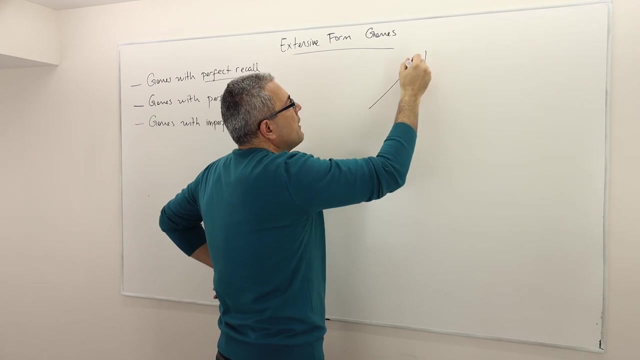 their opponent's previous actions, but they perfectly observe and remember their own actions all right. So meaning, players do not forget anything. That's very important. So this is not a game. This is more like a decision problem. But if you consider this so, player one is acting, choosing between A, B and C. 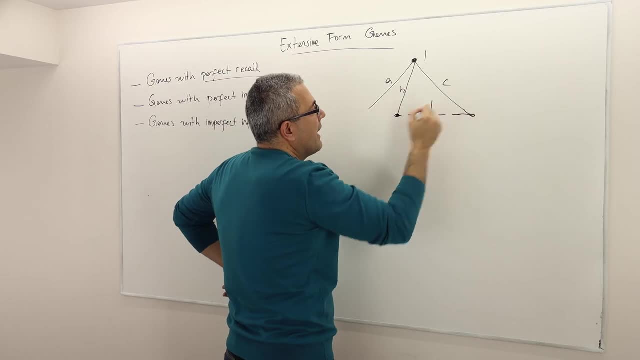 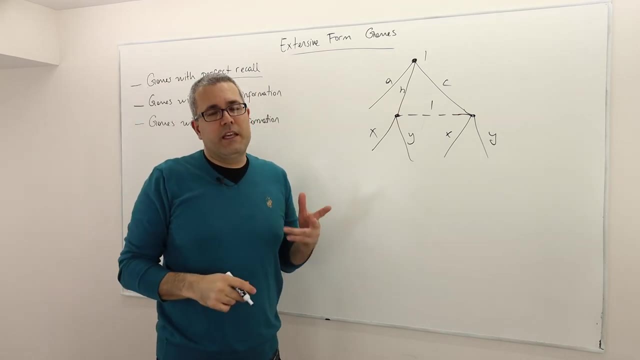 and then later he is choosing again between X and Y. okay, So again, this is not really a game because we don't have a second player. but I mean, if you like, you can make this- you know, more than one person decision problem by adding a second player. 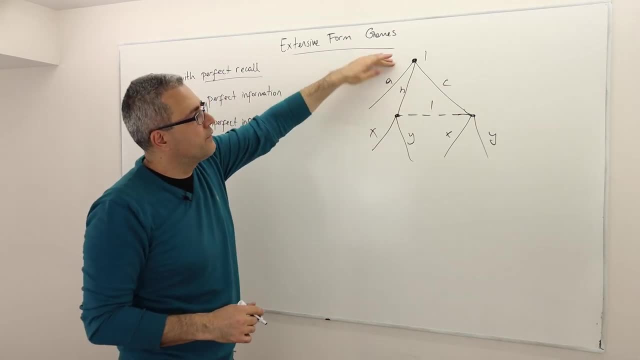 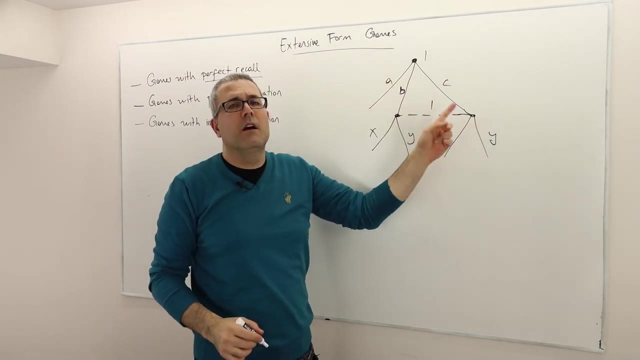 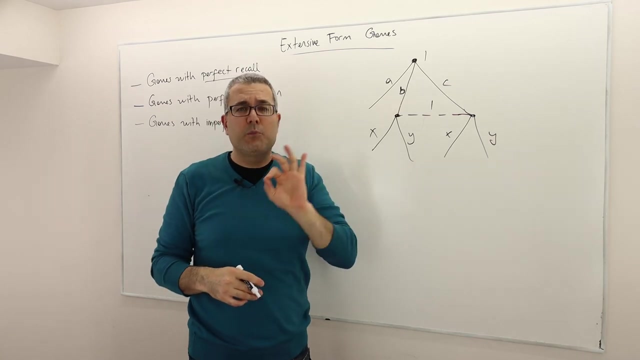 somewhere. But here the idea is the following: The first guy is first choosing A, B and C, but then later he can't remember whether he selected B or C. all right, So he forgets his own action. So we are never going to look at games like this. So each player remembers his. 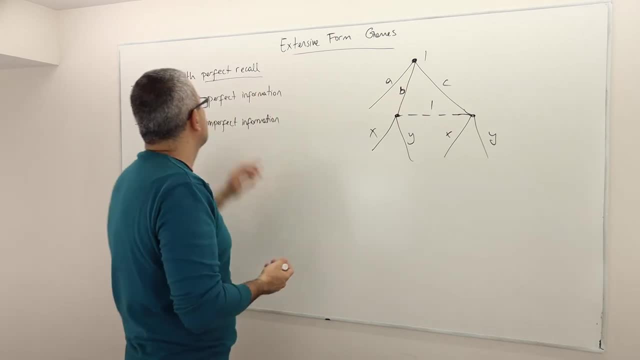 action. So we are never going to look at games like this. So each player remembers his or her action, her own previous actions, all right. so in such games we call perfect recall we know, i mean i know. in reality, by the way, this is not really the case. we make a move and then we forget it. 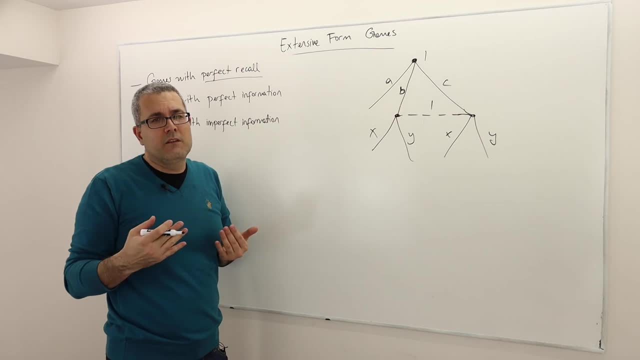 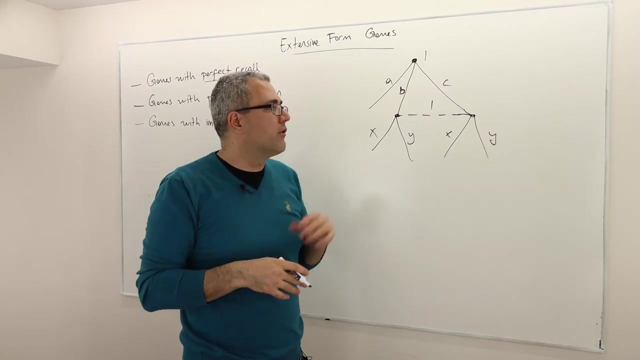 after a while and so we are forgetful in fact, and that certainly influence our sort of behaviors in real life. but the reason we ignore these games are because they cause us sort of interesting technical complications. ariel rubinstein has a very nice paper with michael picchioni, if i am. 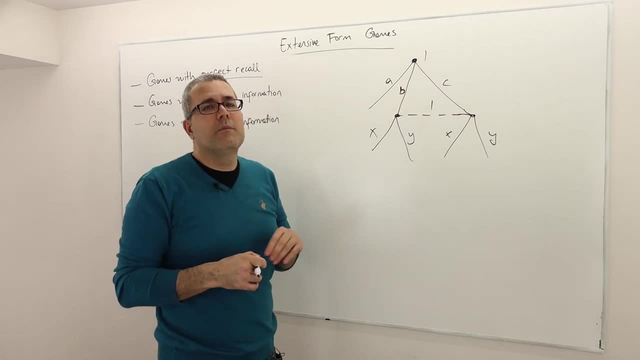 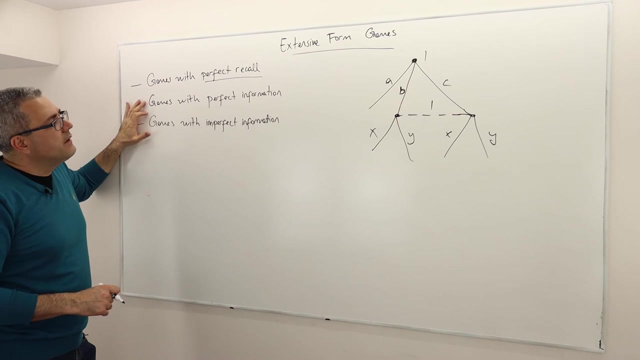 pronouncing his or her name correctly. they are sort of looking at games with imperfect recall. but you know there's a lot of, so it's a. it's a very unfamiliar territory for game theorists, i must admit. all right well, we distinguish extensive form games into two class. 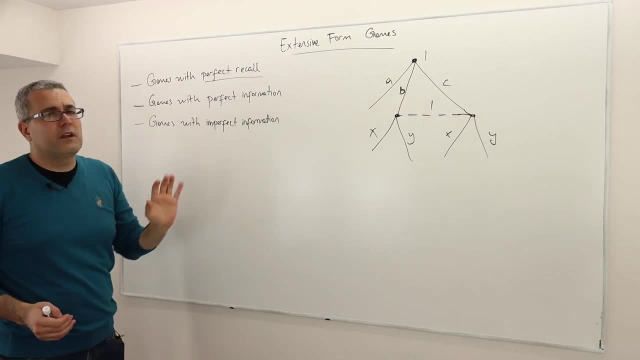 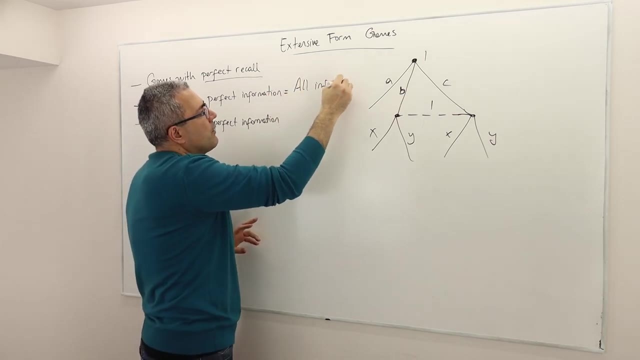 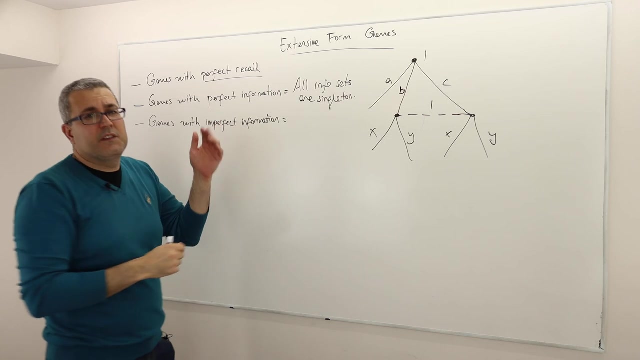 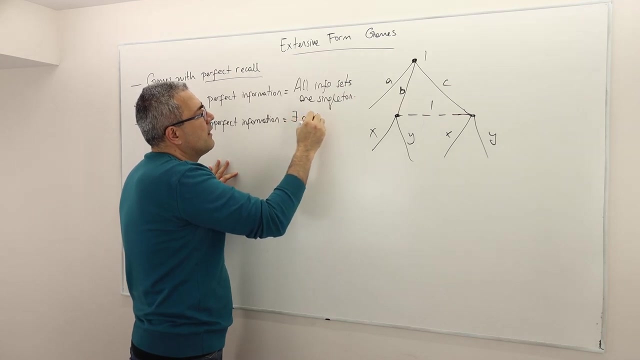 games with perfect information and games with imperfect information. so games with perfect information is basically: all info sets or all information sets are singleton okay, and if this is not true, well then the game is a game with imperfect information, which means there exists at least one information set with. 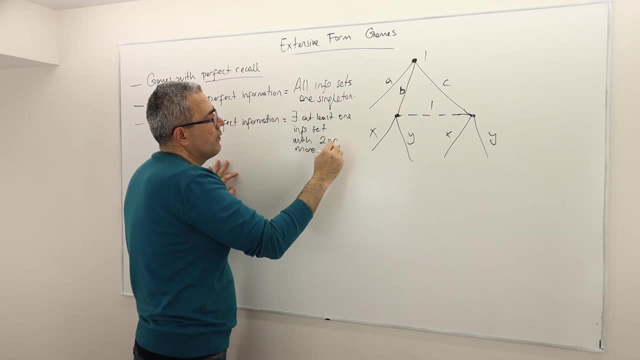 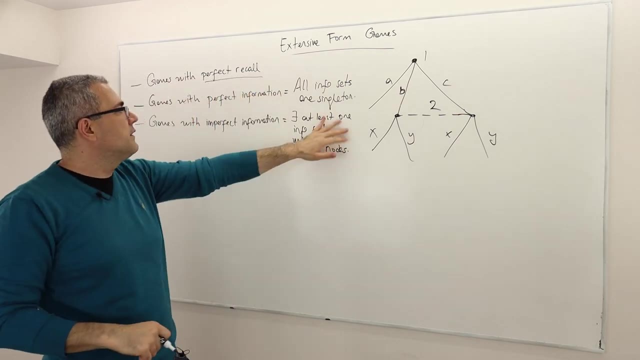 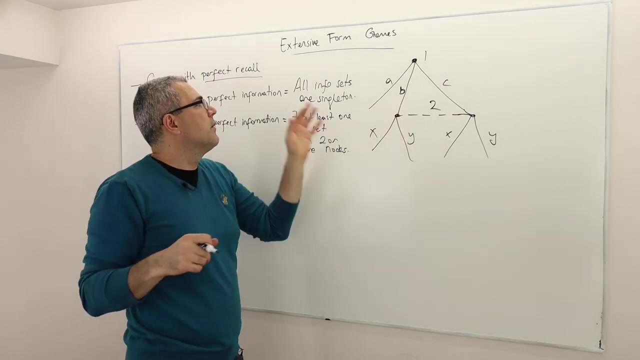 two or more uh, decision notes. okay, so what does that mean? for example, if this is player one, this is player two. this is a perfect recall game, but this is a game with imperfect information, because here in this game there is an information set that is not singleton, so all info sets are singleton means.